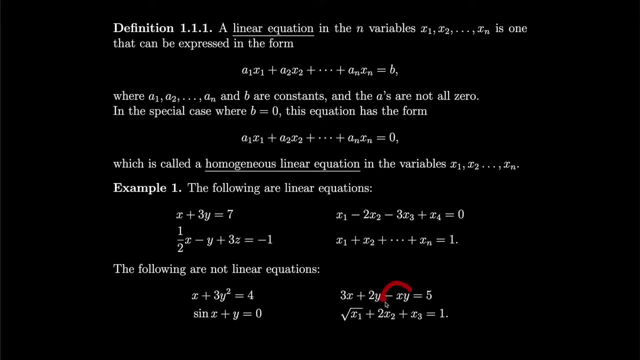 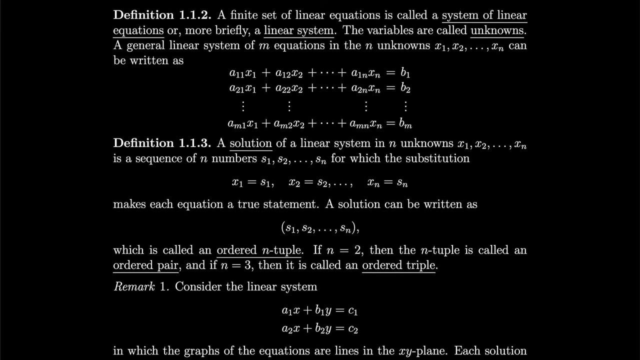 3x plus 2y minus xy equals 5, because we have that product right over here, and square root of x1 plus 2x2 plus x3. because of the square root, A finite set of linear equations is called a system of linear equations, or more briefly: 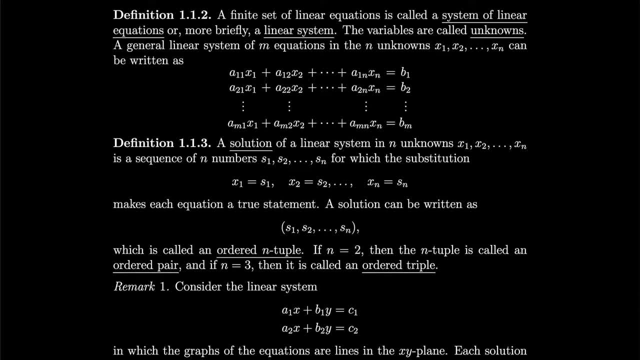 a linear system, The variables are called unknowns, A general linear system of m equations in the n unknowns, x1, x2, through xn, written as this system of equations right over here. So we have each equation on a separate line and then all together. that's our system, where the dots indicate. 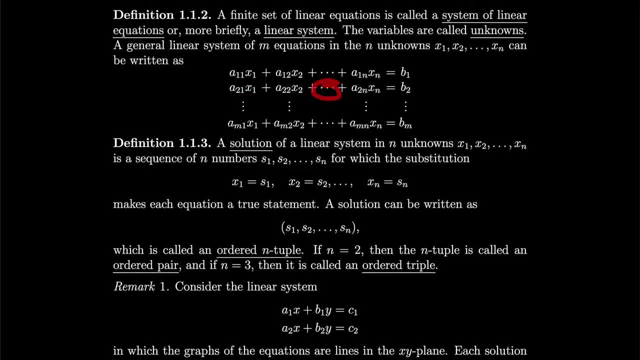 that we're continuing with the equations in between and continuing with the variables in between. Notice that we're using two numbers for indices over here for our coefficients: a1, a12, a1n, where the first number is the row that we're looking at for our equations. This is the first row, so they all have one for the. 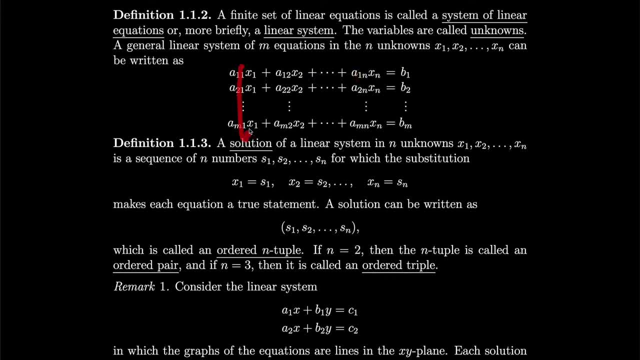 first number and the second number is the column. So this is the first column. second column, nth column: A solution of a linear system in n unknowns- x1, x2, through xn, is a sequence of n numbers, s1, s2, through sn, for which the substitution x1 equals s1, x2 equals s2. 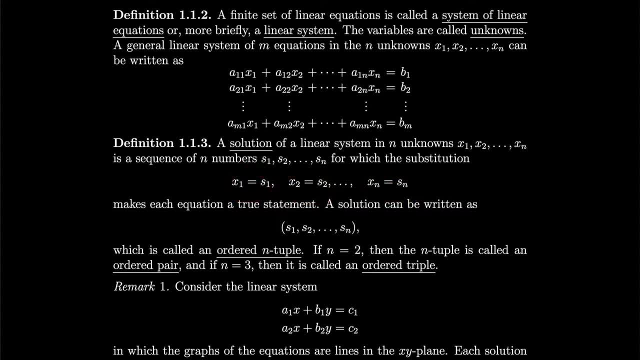 xn equals sn makes these each equation a true statement. A solution can be written as s1, s2 through sn, which is called an ordered n-tuple. If n equals 2, then the n-tuple is called an ordered pair, and if n equals 3, then 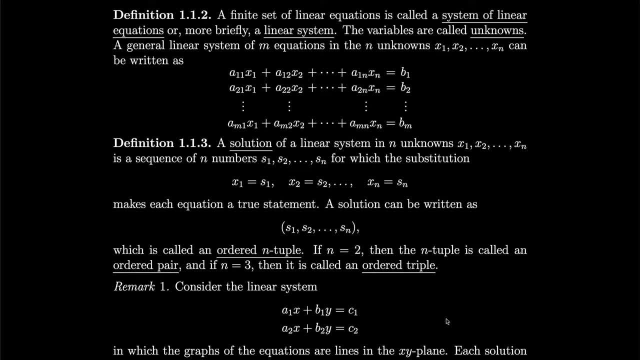 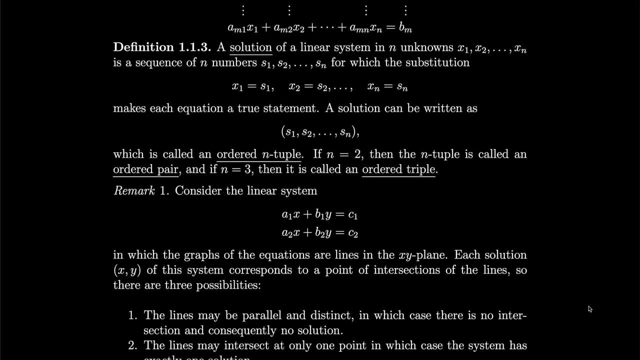 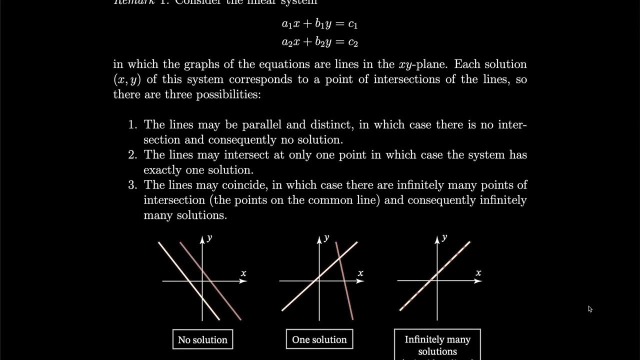 it is called an ordered triple. Consider this linear system right over here, in which the graphs of the equation effluent, xn plus the variable a1.. are lines in the x-y plane. Each solution x-y of the system corresponds to a point of intersection of the lines. so there are three possibilities. Our first: 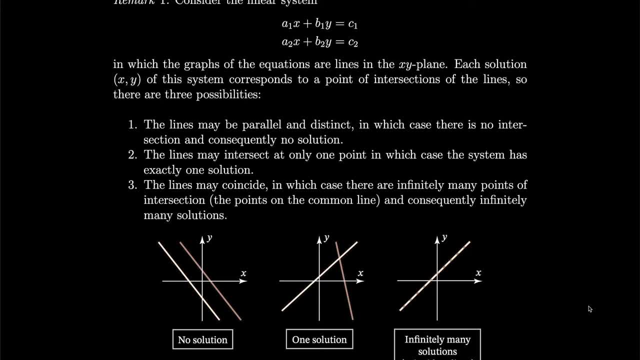 possibility is that the lines are parallel and distinct, in which case there is no intersection and consequently no solution. Our second possibility is that the lines may intersect at only one point right over here, in which case the system has exactly one solution right over here. 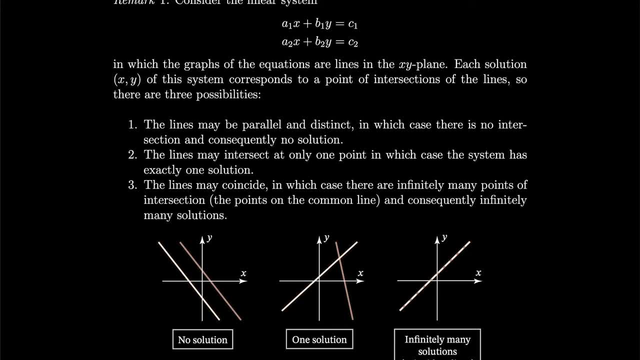 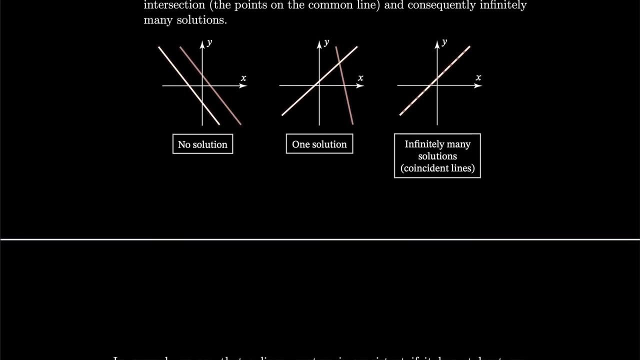 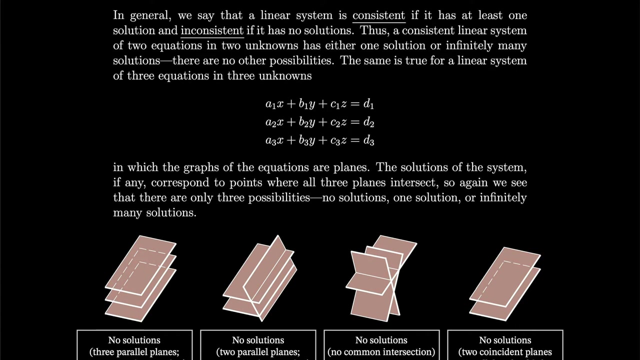 Third possibility is that the lines coincide, so we have one line and then another line right on top of it, in which case there are infinitely many points of intersection, the points on the common line, and consequently infinitely many solutions. In general, we say that a linear system is consistent if it has at 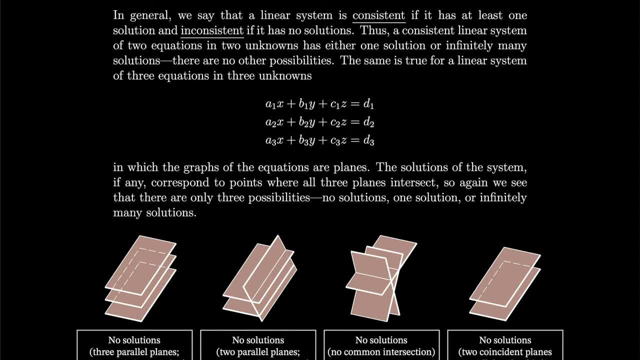 least one solution and inconsistent if it has no solutions. thus a consistent linear system of two equations in two unknowns has either one solution or infinitely many solutions. There are no other possibilities. The same is true for a linear system of three equations and three unknowns in 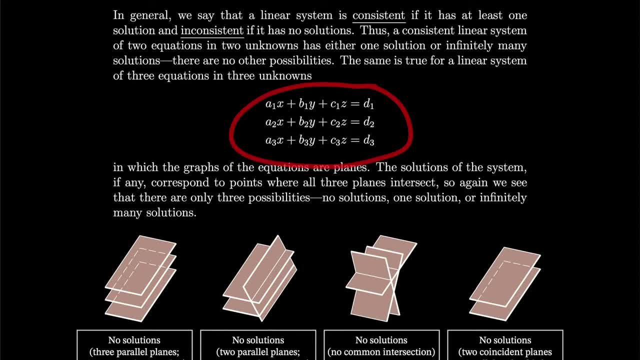 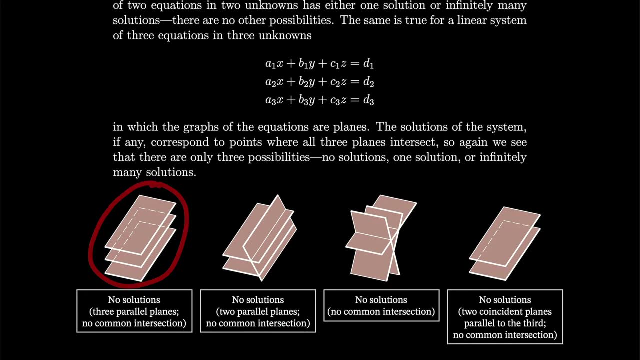 which the graphs of the equations are planes. The solutions of the system, if any, correspond to points where all three planes intersect. so again we see that there are only three possibilities: No solutions, one solution or infinitely many solutions. So either we have these planes, that they're just kind of stacked, 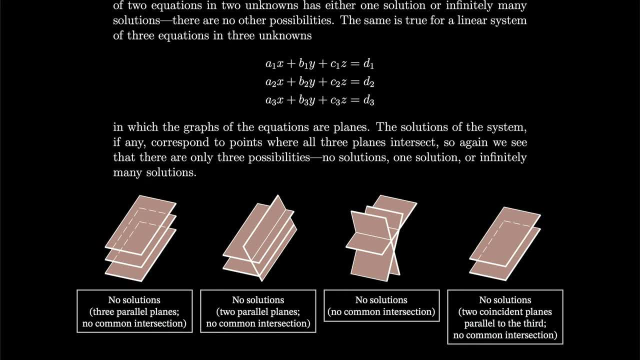 on top of each other or left to right, doesn't matter. or we have these two parallel planes. notice, this one over here and this one underneath it over here. don't touch. so even though they touch, they both touch this one. they. 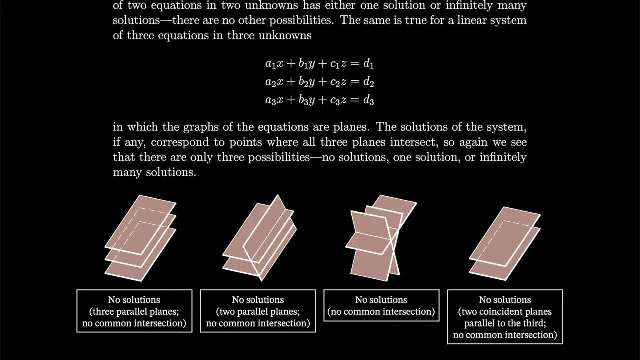 don't all touch together in the same place, so there is no solution In this case. they all touch two other planes. this one touches over here, over here and over here, but they do not meet in the middle. so no solution. 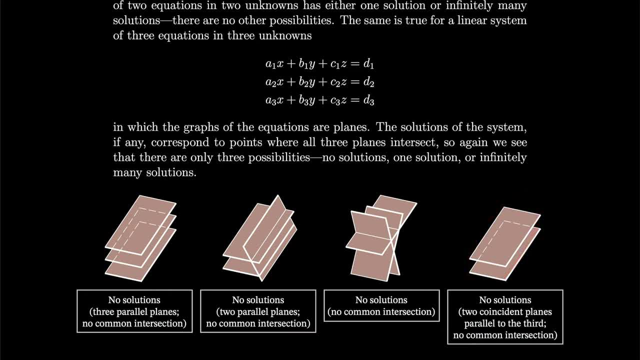 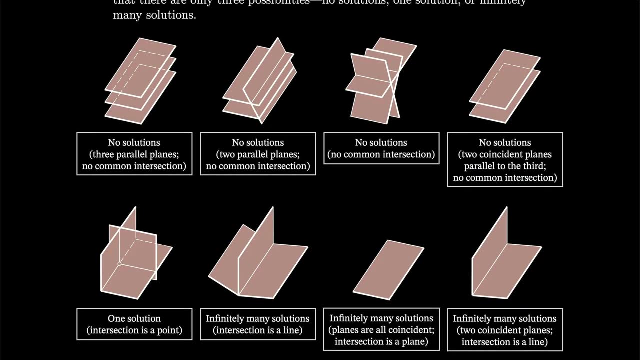 Over here. we have two planes, let's say over here- which both lie right on top of each other. they coincide, so there's no solution because the other one does not. Over here we have one solution because they all intersect in the same. 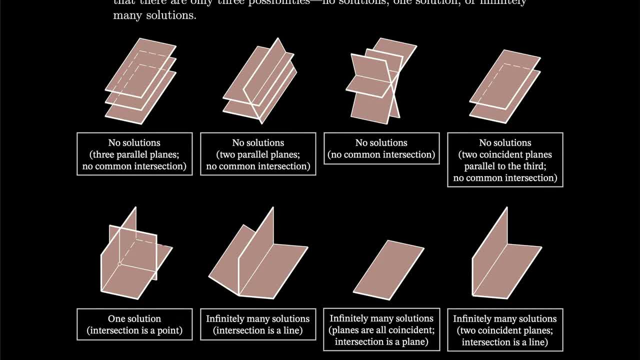 place and over here we have infinitely many solutions because they all intersect in the same place infinitely many times. across this line, Over here, all three planes are stacked literally just all together, so they coincide. infinitely many solutions, and over here we have infinitely many. 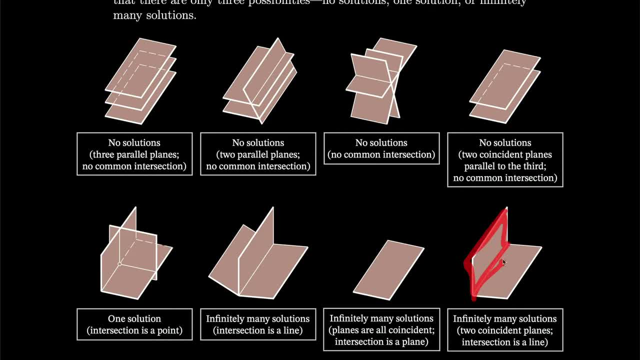 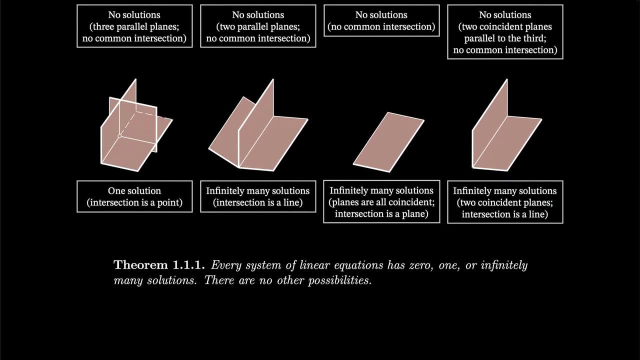 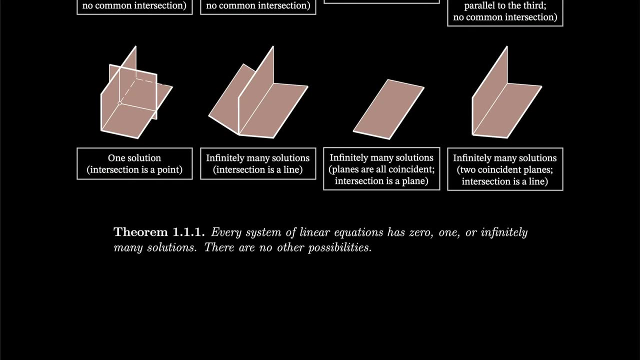 solutions because two of the planes coincide, let's say these two and then the third one intersects right over here in this line. Every system of linear equations has zero, one or infinitely many solutions. there are no other possibilities. We're not going to prove that, but we are going to use that quite extensively. 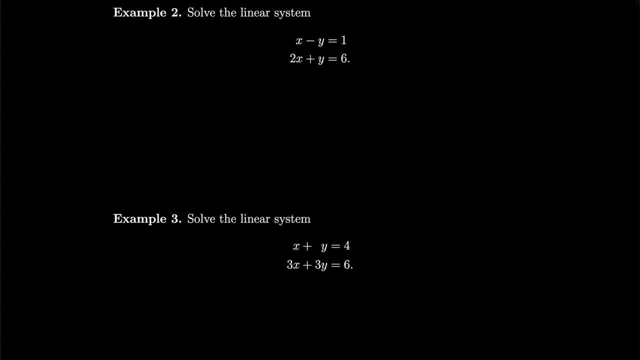 So, as an example, how about we solve this linear system right over here? x minus y equals 1,, 2x plus y equals 6.. What we can do is multiply the top equation by minus 2, and we'll just add that to the second equation, So we'll end up with x minus y. 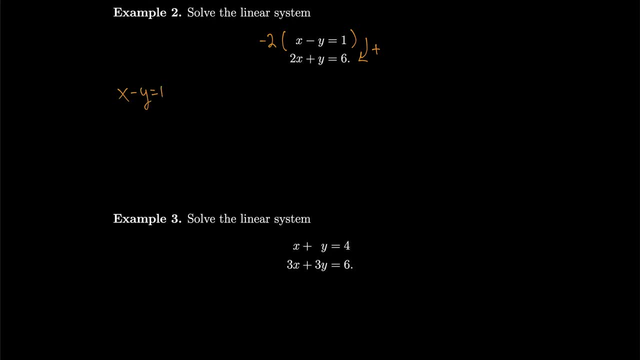 equals 1.. Even though I said I was more multiplying it by negative 2 and adding it to the second one, I'm going to leave the top equation the same. I'm only multiplying it by negative 2 in my head and adding it to the second one. so I'm only going to change the second one. So 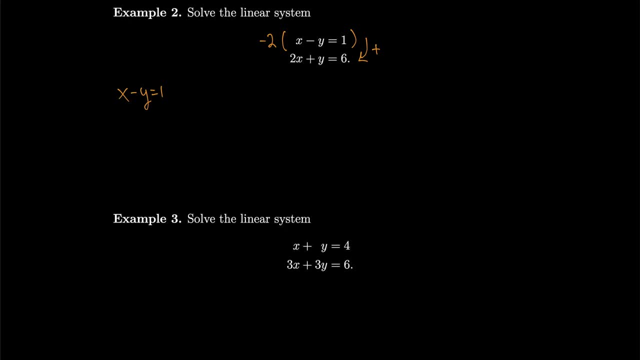 when I multiply the top by negative 2, I get negative 2x plus the 2x in the bottom. so there's 0 over here. but I'm not going to bother writing 0. I'll just leave it as nothing, because when I take the negative 2 and I multiply it by the, 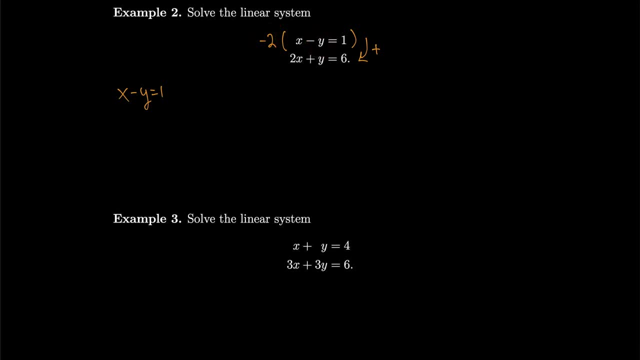 negative y, I'll get a positive 2y plus the 1y will give me 3y, so I get 3y equals. well, it's not 6 anymore, because I had negative 2 times. 1 is negative 2,. 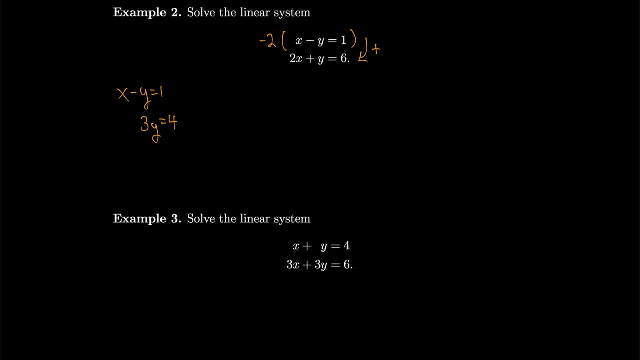 so negative 2 plus 6 gives me 4.. Okay, so now I've simplified things a little bit because I've completely eliminated the X from the bottom equation. So if I once solve the bottom one for Y I now can, I'll divide by 3 on both sides and get the y is 4.9.. 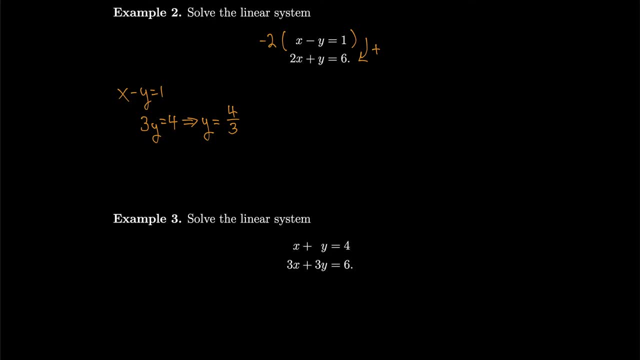 thirds. So now I can go back and plug in for x. I'll see that x is 1 plus y. by just moving over this y, add it to both sides, I get x is 1 plus y. So that means that it's going to be 1 plus 4 thirds, because I already know what y is. I just 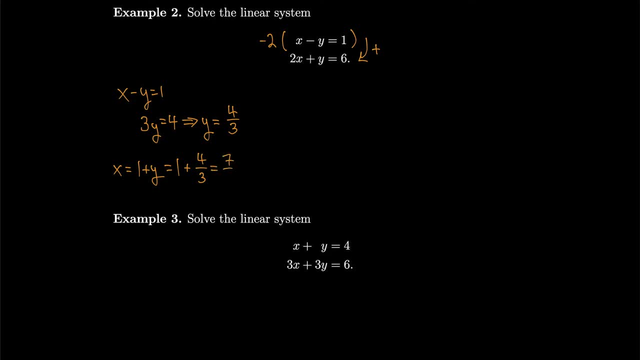 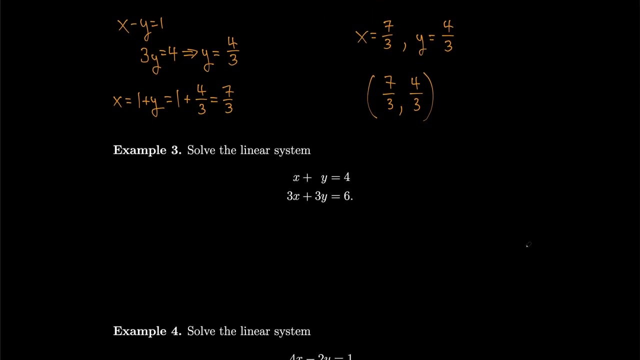 solve for it. So that's 7 thirds. Okay, so now we know that x is 7 thirds and y is 4 thirds, So our solution is the ordered pair: 7 thirds, 4 thirds. Let's do another example. How about we solve this linear system? x plus y equals 4, 3x plus 3y. 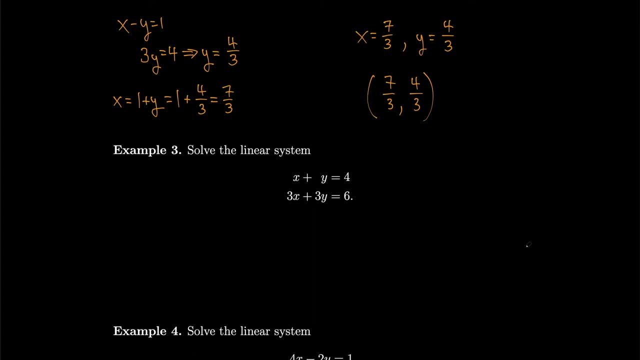 equals 6.. So what I can do is rewrite the top: x plus y equals 4.. I will take the top, multiply by negative 3, add it to the bottom. Notice what will happen. Negative 3x plus 3x is 0. The negative 3y plus 3y will also be. 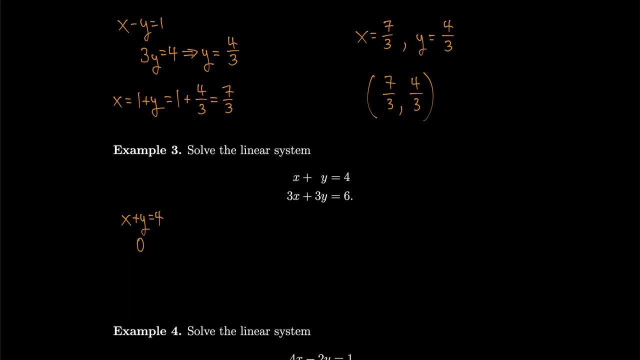 0. So I'll just write 1, 0. And then if I take negative 3 over here, I'll get negative 12 when I multiply on this side. So negative 12 plus 6 will give me negative 6.. So 0 is never equal to negative 6.. So there's no solution. 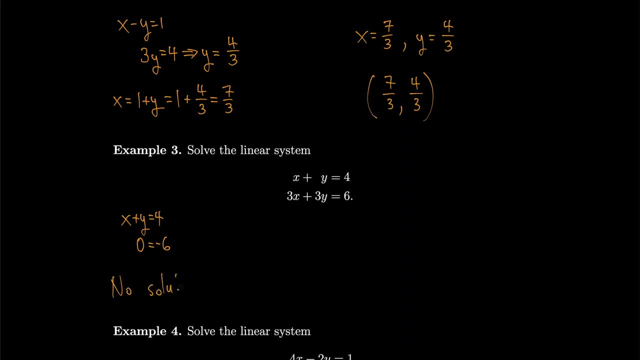 So there's no solution. Notice, if we were to graph this, it would look something like this: Here's my y-axis, Here's my x-axis. Here's, let's say, x plus y equals 4.. And then over here could be: let's. 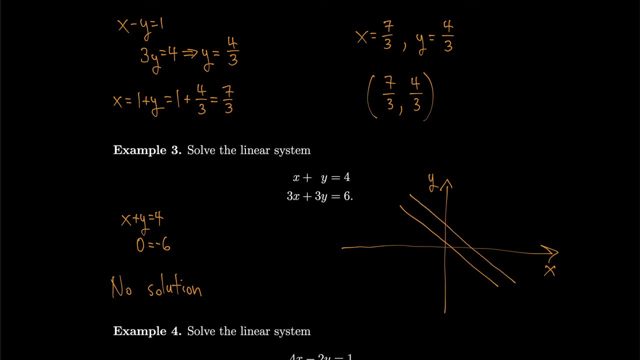 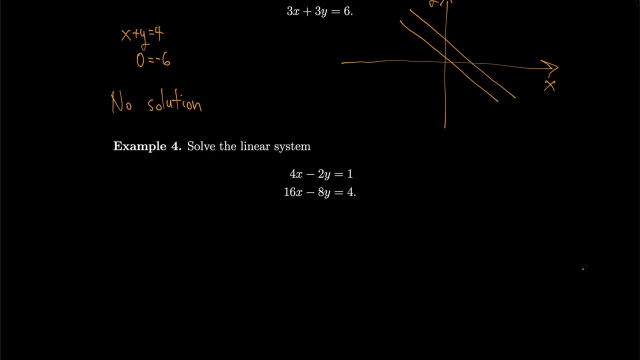 say: 3x plus 3y equals 6.. Notice: they do not coincide or intersect in any way, which is why we get no solution. Okay, Okay, Okay, Okay, Okay. How about we try solving this one? We have: 4x minus 2y equals 1.. 16x minus 8y equals. 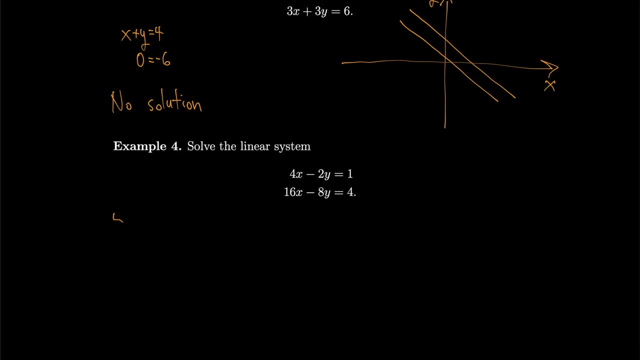 4.. So, again, we'll rewrite the top. We have 4x minus 2y equals 1. And we won't always rewrite the top. It just happens to be more convenient in this case to manipulate the top and add it to the bottom, one each time for these particular examples that we've been. 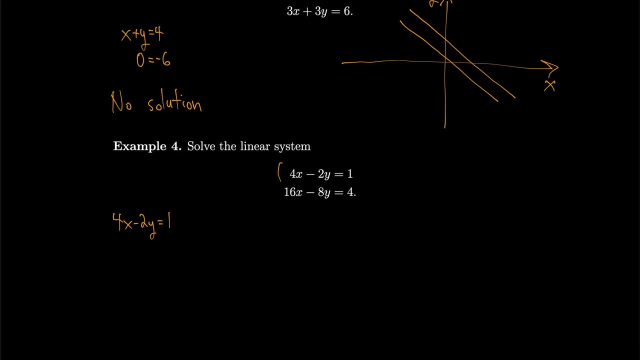 doing. Notice, though, when I take negative 4, I get negative 4.. And then I get negative 4 times the top and add it. I'm going to end up with 0 here, 0 here. So I just have. 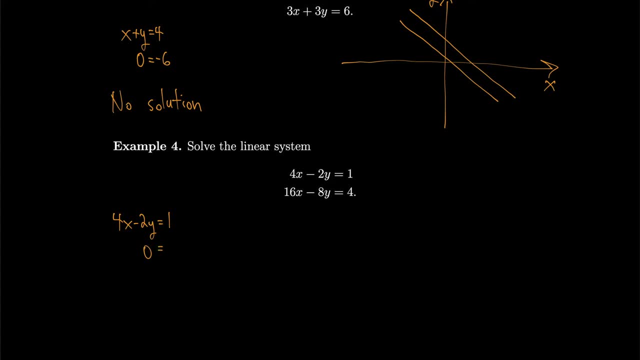 0 on the left again. However, this time negative 4 is what this one will become. Add it to 4.. I'll get 0 on the right also, But that's great, because 0 is always equal to 0. So in. 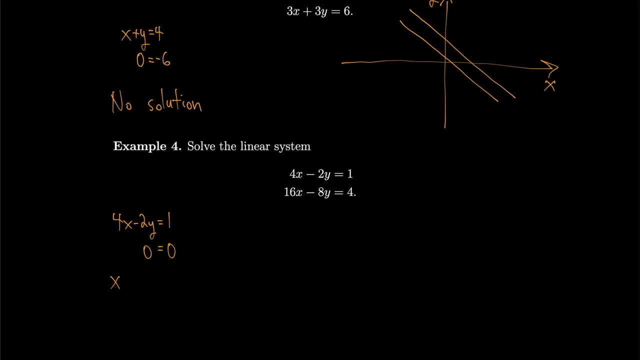 this case. I've got lots of solutions, Infinitely many actually. I'll have x equals. well, I can solve by adding 2y to this side, divide by 4.. So I'll get 1 fourth plus half y. So 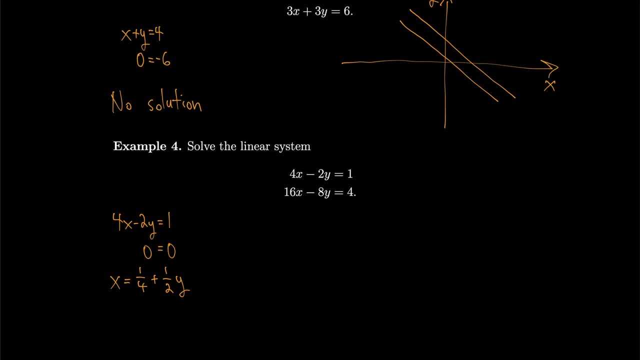 instead of writing x in terms of y, what I can do is I can change y to another variable called a parameter. I'll say t. Okay, So x equals 1 fourth plus half t, And we'll say that y is equal to t, So functionally, 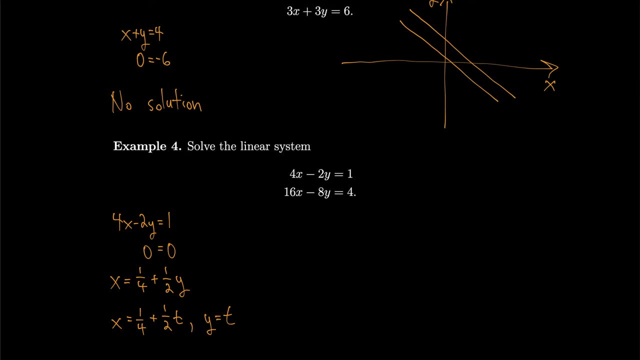 there isn't really any difference here in our answer. It's still the same answer. I just replaced y with t. I only do this because, as we're going to see later on, sometimes it's more convenient to insert a parameter like this when interpreting our answers. Kind, 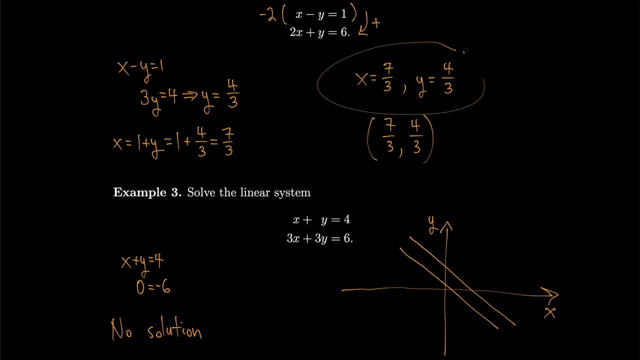 of like how over here I wrote: you know, x equals 1 fourth plus half t. So x equals 1 fourth plus half t Here. I wrote this for our x and y values, but I wrote this also for our solution. Both of these are equivalent, just two alternative ways of representing. 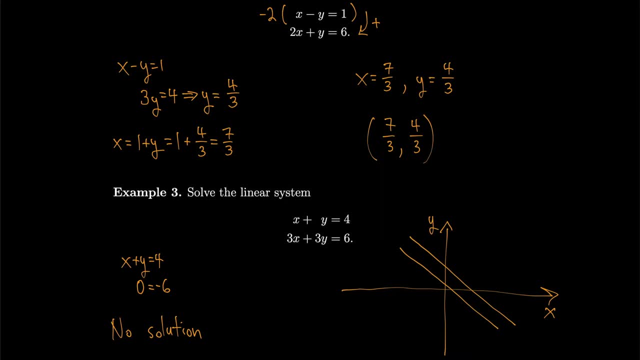 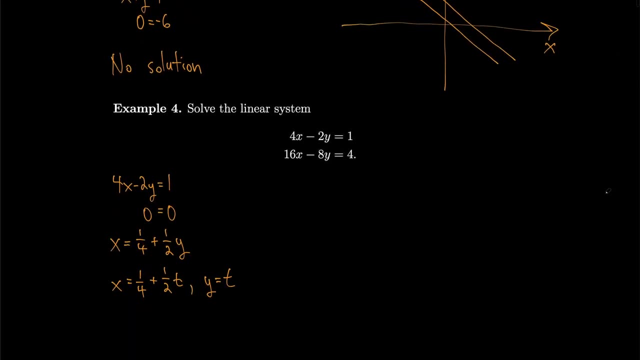 it. We just use whichever one is more convenient for the particular problem that we're doing. And right now we're just at the beginning, so we're trying to learn as many different ways of representing our solutions as possible. So just to take a look at what this graph: 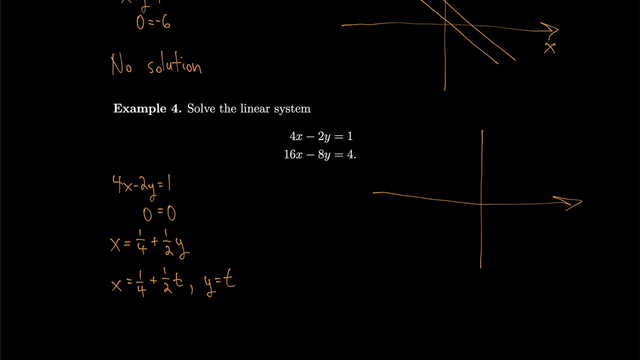 might look like: Here's let's say x, Here's y, here's my line, and right on top of it is the other equation. So I have, for example, different values of my parameter. t, which is equal to y, will give me different. 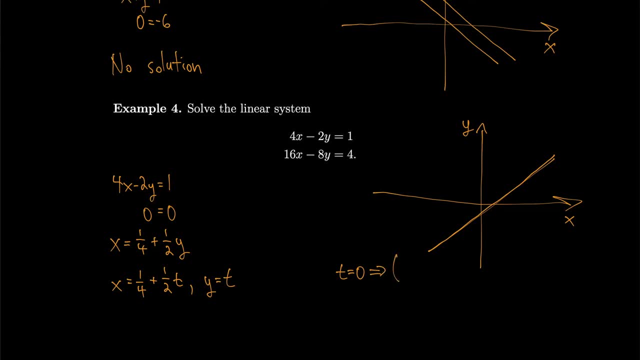 solutions. If t equals 0, I'll plug in 0 for y or t, if I'm using this, and I'll see that I have 1 fourth 0.. So I have 1 fourth 0.. If t equals 1, then I would have 3 fourths 1 as a solution If t is equal to minus 1,. 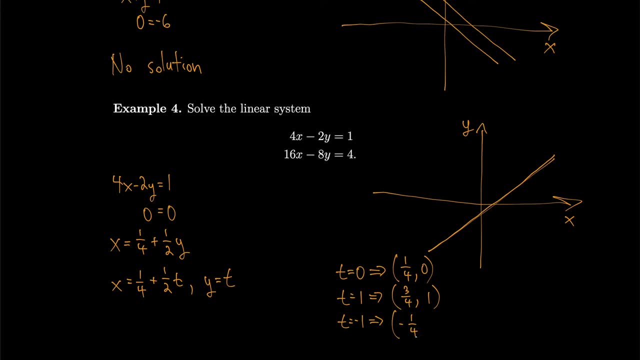 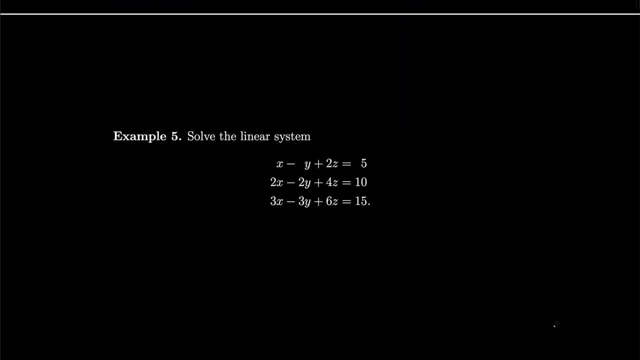 then I end up with negative 1, fourth negative 1 as a solution, And you can do that for infinitely many values of t. Okay, how about we solve this linear system? Okay, Okay, Okay. so here's the linear system now. So we have 3 equations. How about I take this? 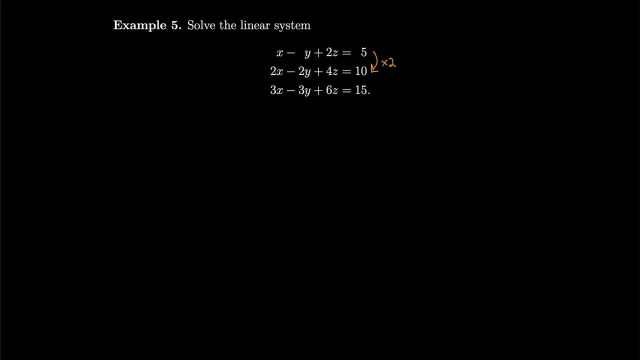 one. multiply it by 2, add it there, because that way I'll get the 5 into the 10. I can get 5 to match up with 15 by multiplying this by 3. So if I do that and subtract them, 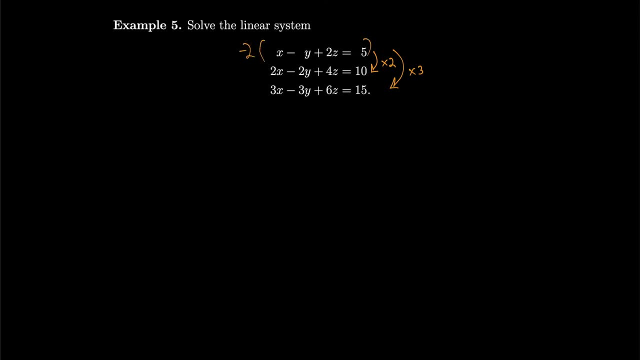 or you could think of it as multiplying this by negative 2 if you like thinking of it that, that better. then I can eliminate the bottom two variables for x, and actually it looks like it's going to match up for y and z also. So for the top I should get: x minus y plus 2z equals 5. 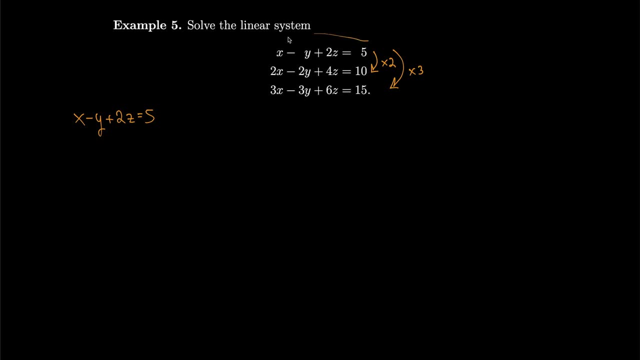 and when I multiply this by 2 and subtract it from this, then I should get 0 for the x, 0 for y, 0 for z. So just get 0, and then I end up with 10 minus 10 is 0. 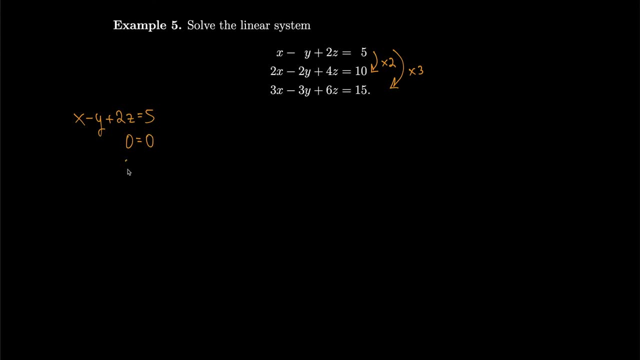 and it looks like the same thing for the bottom equation when I multiply by 3.. So if I want to solve for x, I'll move everything else over and I'll get that x equals 5 plus y minus 2z. So again, I'll parametrize and I will replace y and z. 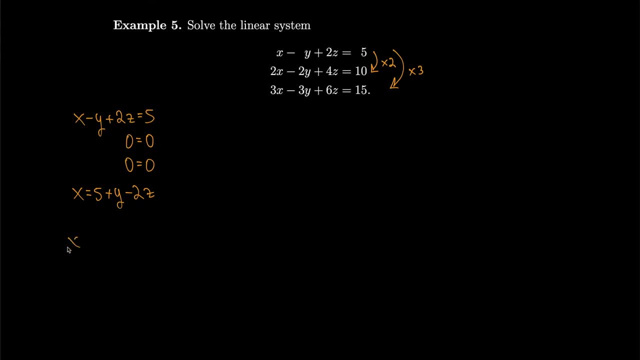 with two other variables. How about let's say r and s? So x equals 5 plus r minus 2s, and I'm going to set y equal r, z equals s. Those will be my parameters instead of y and z. So this way I can look at all sorts of different values of my parameters and see what different 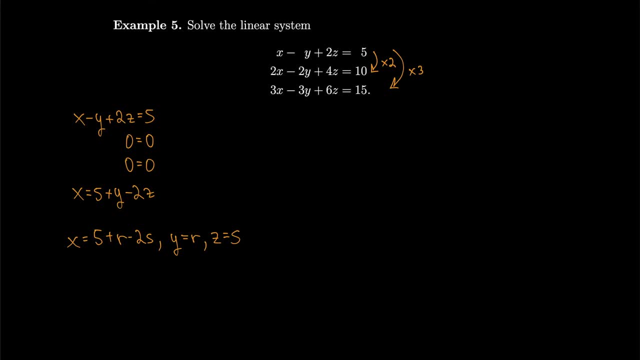 solutions I get So. well, let's take a look at a graph. So let's take a look at our solution set. Let's see, and the x, y, z plane should be something like this: and it's just the plane: x minus y plus 2z equals 5.. So I should get something roughly. 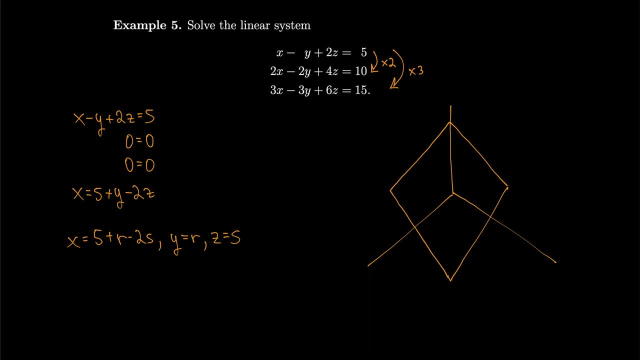 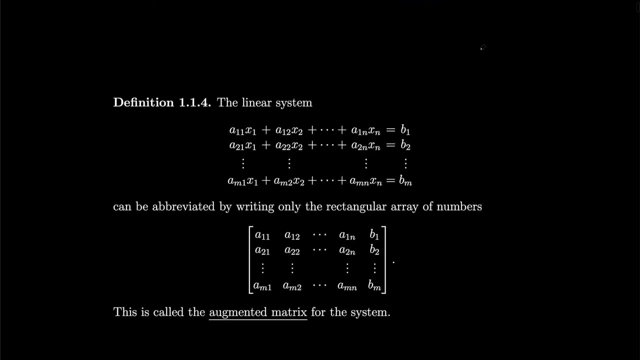 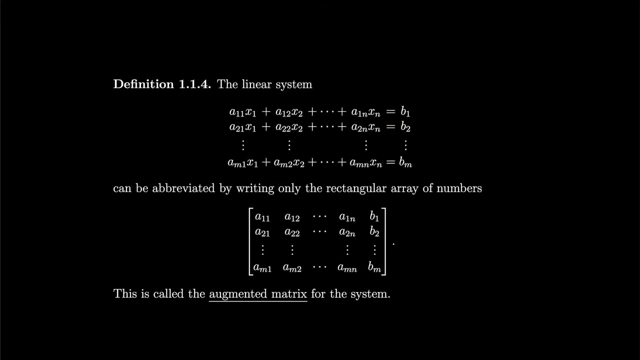 like this and the solutions are just everything in this plane over here. So, for example, if I took, say, r equals 1 and s equals 0, then I would get the solution 6, 1, 0. The linear system a1, x1, a1 and 2, x2 and so on to equal to b1, and then a21, x1,, a22, x2 to equal. 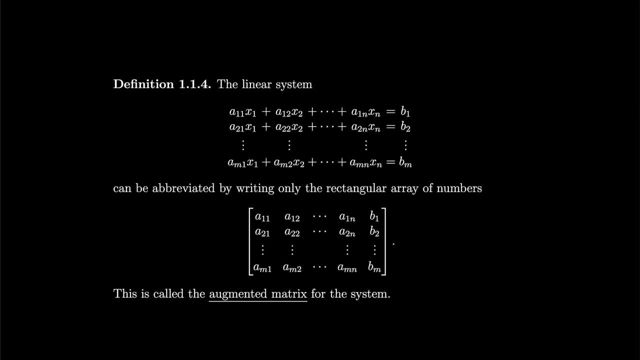 to b2 through am1, am2, x2, amn x2.. So I could get the solution 6, 1, 0.. So I took a1, x1, a1 and 2, x2 and so on to equal to b1, and then a21, x1,, a22, x2 to equal to b2 through am1, am2, x2, amn x1. 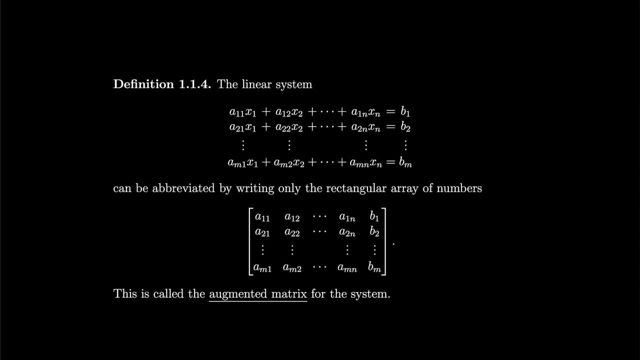 n equal bm can be abbreviated by writing only the rectangular array of numbers, that's the coefficients for each of the variables. so i just pull off the a11, the a12 and so on, and then i don't have to write all these variables, it's just assumed that they're there. we call this the. 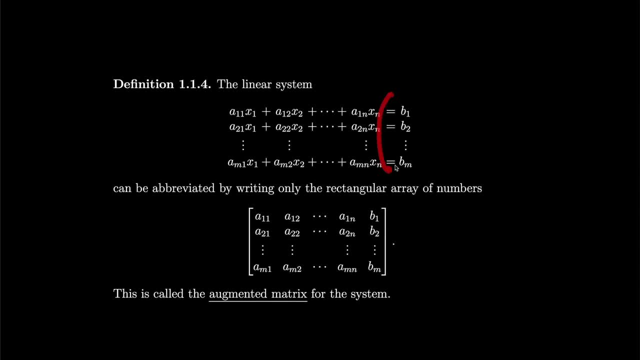 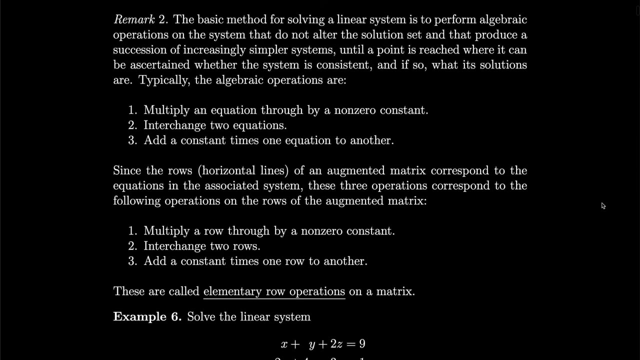 augmented matrix for the system. notice: we don't even have to write any equal signs or any pluses, because it's just a simpler way of writing or help a whole system that uses, you know, less ink. the basic method for solving a linear system is to perform algebraic operations in the system. 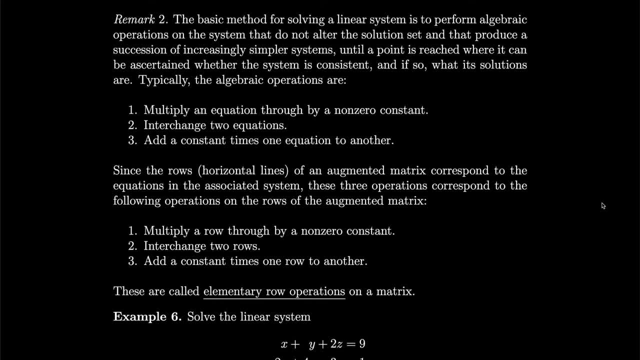 that do not alter the solution set and that produces succession of increasingly simpler systems until a point is reached where it can be ascertained whether the system is consistent and, if so, what its solutions are. typically, the algebraic operations are: to multiply other an equation through binon, zero, constant. to interchange two equations, to add a. 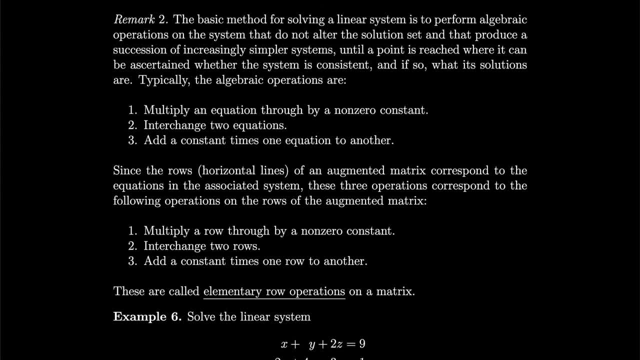 constant times one equation to another, and since the rows, the horizontal lines of an augmented matrix, correspond to the equations in the associated system, these three operations correspond to the following operations: on the rows of the augmented matrix, We can multiply a row through binon zero constant, because 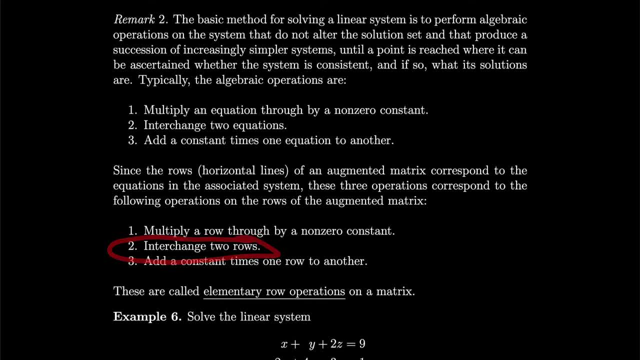 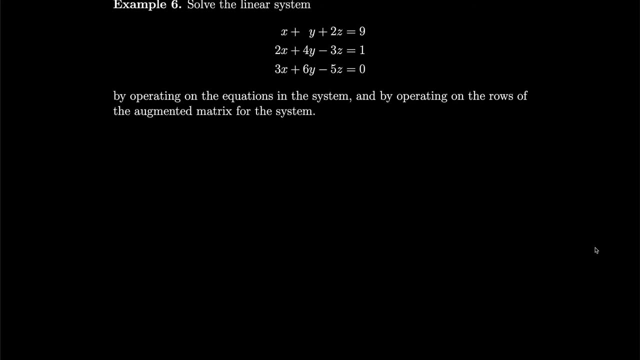 the row is an equation. we can interchange two rows, we can add a constant times one row to another, and these are called elementary row operations on a matrix. Let's do an example and solve the linear system: x plus y plus 2z equals 9, 2x plus 4y minus 3z equals 1, 3x plus 6y minus 5z. 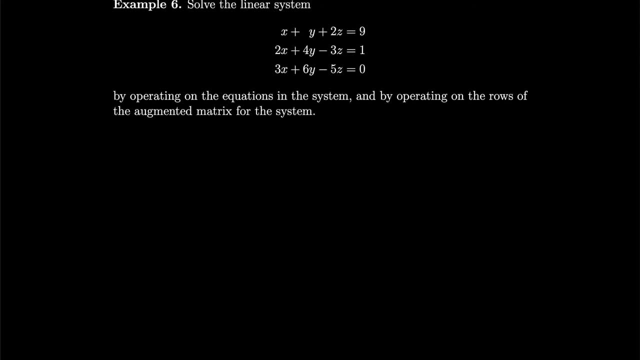 equals 0, by operating on the equations in the system and by operating on the rows of the augmented matrix of the system. So we'll do both methods at the same time. So first I'll rewrite it: x plus y plus 2z equals 9,. 2x plus 4y minus 3z equals. 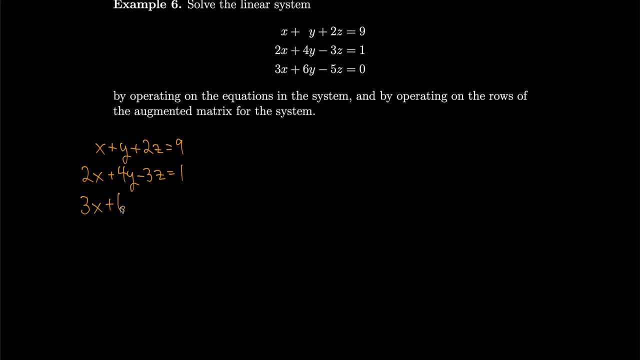 1, and 3x plus 6y minus 5z equals 0. The augmented matrix for that system will just be the coefficients of each of the variables. so for our top equation we have 1 as the coefficient for x. 1 is the. 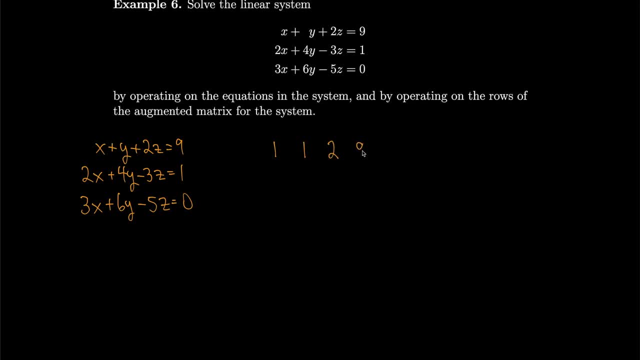 coefficient for y, 2 is the coefficient for z and 9 is what it equals. Then we end up with our second row for a second equation of 2, 4 minus 3, 1, and then our last one is 3, 6 minus 5, 0, and that's our augmented matrix. So we're going to. 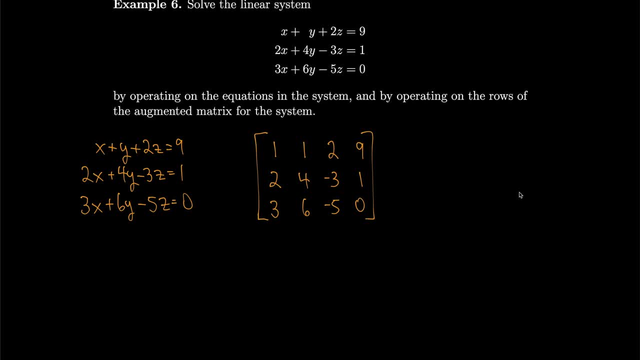 manipulate our equations and our matrices at the same time. So how about we rewrite: x plus y plus 2z equals 9.. What I'm going to do is I'm going to add negative 2 times the first row to the second. I'll end up with 2y. 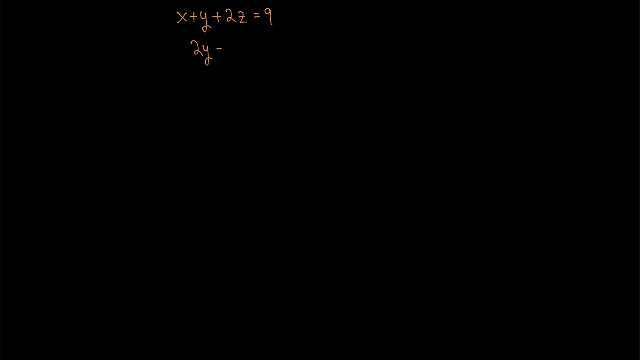 minus 7z- oops, that's not a 7,, that's a 7, equals negative 17.. Notice, all I did was take negative 2 times this equation and add it to this equation over here, so my x cancels out entirely. 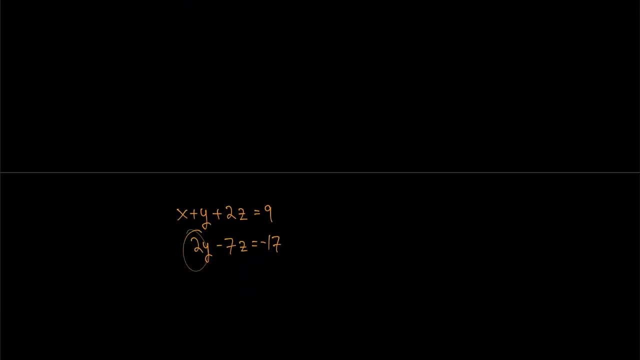 Negative. 2y plus 4y gives me the 2y Negative 2 times 2z is negative 4z plus negative 3z is the negative 7z and negative 2 times 9 is negative 18, plus 1 is negative 17.. 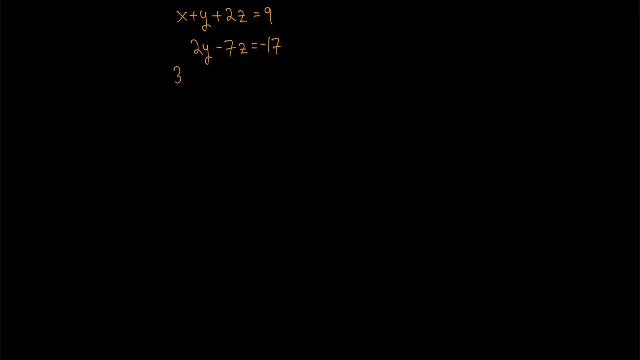 So that works out: 3x plus 6y minus 5z equals 0.. And my matrix, my augmented matrix, would be 1, 1,, 2,, 9,, 0, 2, minus 7,, minus 17,, 9, 9,. 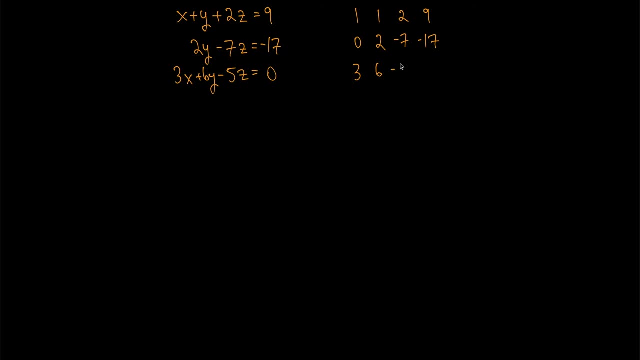 6, negative 5, 0.. And for my next step, I'll rewrite the top equation again: x plus y plus 2z equals 9.. I'll leave the second equation the same too: 7z equals negative 17.. 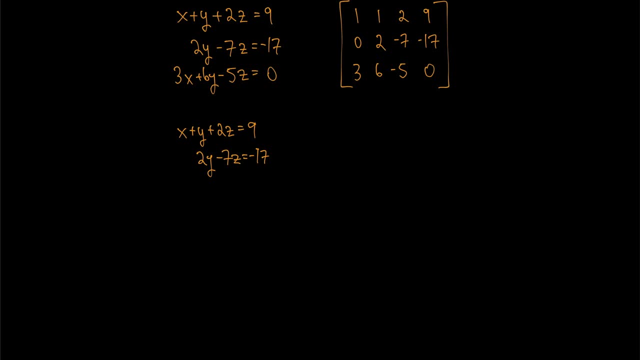 But then I'm going to try to eliminate x. now for my third equation. There's a 3x in the bottom, so I'll multiply the top by negative 3, and I'll get 3y minus 11z equals negative 27.. 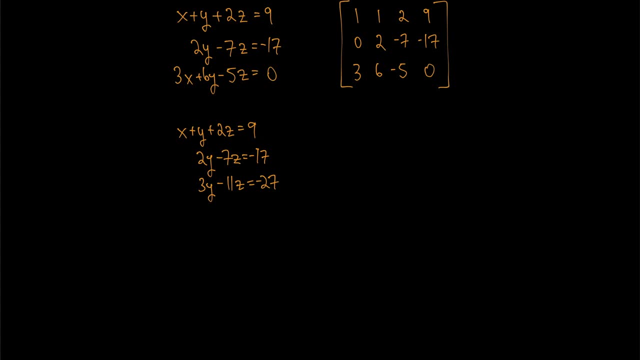 So I just took negative 3 times this and added it to this, Or you can think of it as this minus 3 times this. So I end up with 1, 1, 10.. That's it, Thank you. 1, 2, 9,, 0, 2, minus 7, minus 17, and 0, 3, minus 11, minus 27.. 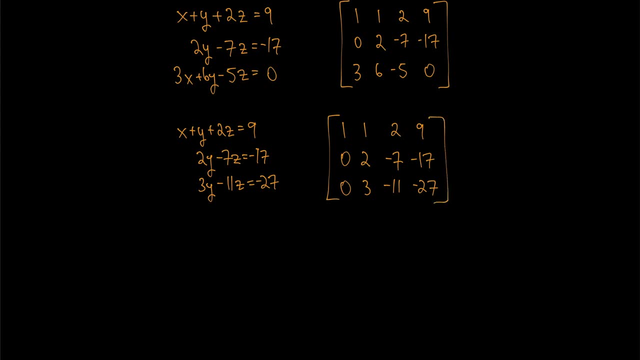 Notice that for each of these operations I didn't actually have to operate on this system. I didn't have to actually take those equations and do it. I could have just worked with the numbers in my matrix If I just take this entire top row times negative 3 and add it to this row. 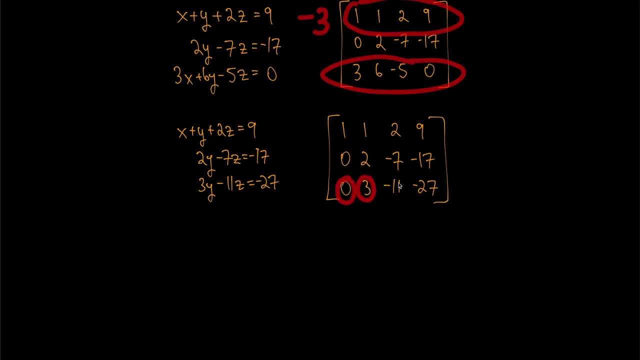 then I end up with 0 over here, I end up with 3 over here. negative 11 over here. negative 27 here. It's exactly the same as this side, So I don't actually have to write all of this in general. 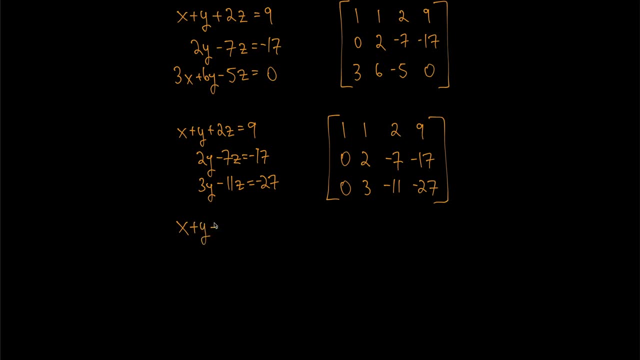 For our next step, we'll rewrite the top again. x plus y plus 2z equals 9. And I'm going to try to get y by itself, so I will divide by 2 or multiply by 1⁄2,. 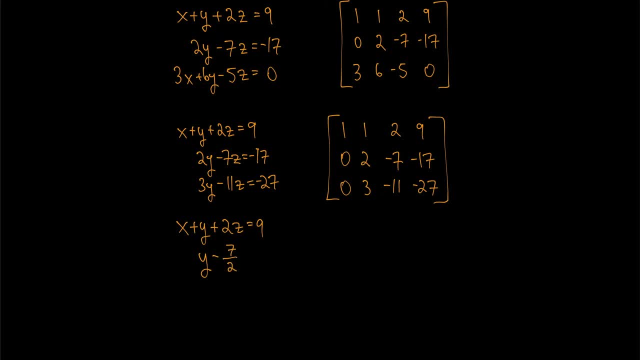 however you like to think of it. So y minus 7 over 2z equals negative 17 over 2.. And I'll leave my bottom equation the same: 3y minus 11z equals negative 27.. So my matrix is 1.. 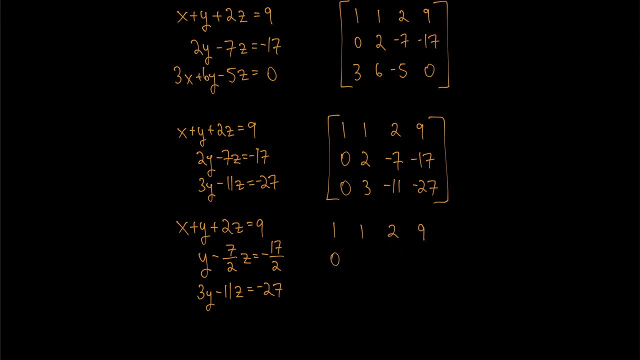 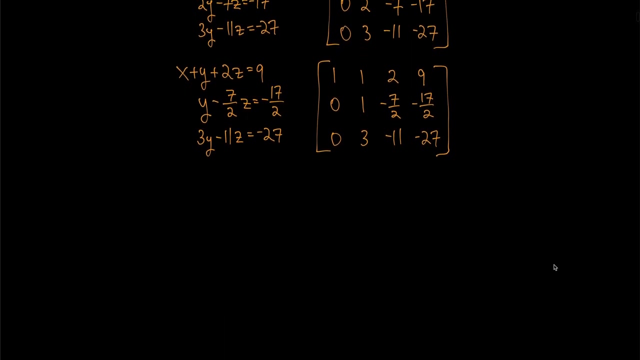 1, 2, 9,, 0, 1, negative, 7 over 2, negative, 17 over 2, and 0, 3, negative, 11, negative 27.. Let's keep going. I'm going to now take my. 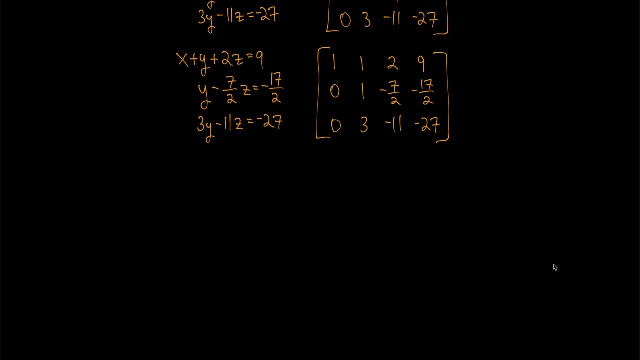 last equation and I'll take negative 3 times this. that way I can eliminate the y in the bottom row, So I'll get x plus y plus 2z equals 9.. y minus 7 over 2z equals negative 17 over 2.. 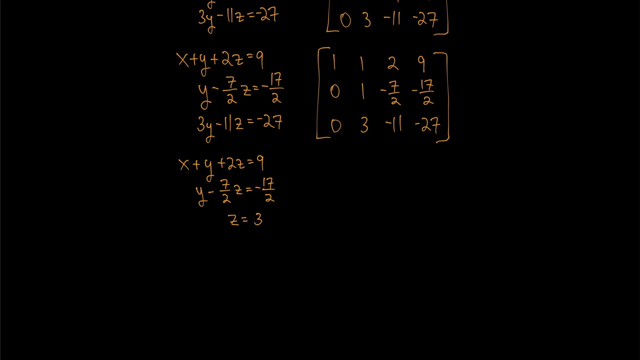 And z equals 3.. And then that will give me 1, 1,, 2, 9, 0, 1, negative 7 over 2, negative 17 over 2, and 0, 0, 1, 3.. 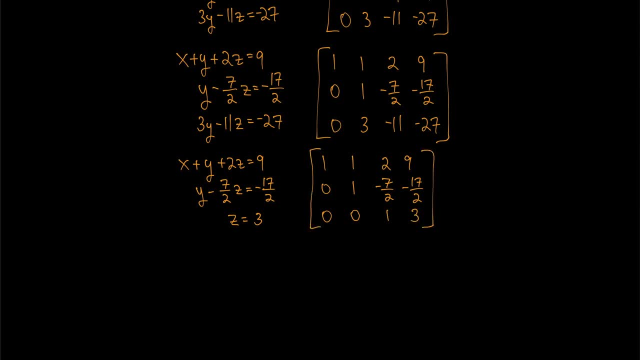 So we figured out what z is. That's great, Great. How about we now try to get rid of y in the first equation? That way we can only have y in one of them. So we'll add negative 1 times the second equation to the first equation. 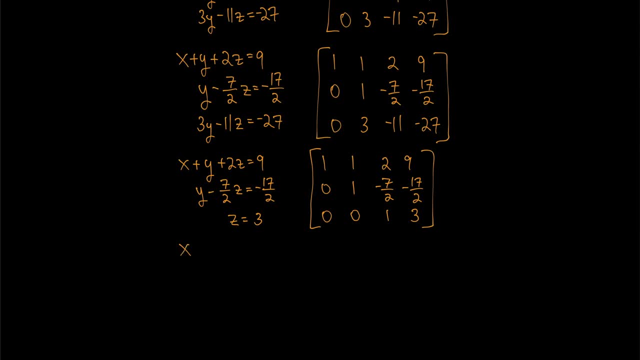 So I'll end up with: x plus 11 over 2z equals 35 over 2.. So I'll get: y minus 7 over 2z equals negative 17 over 2, and z is still 3.. So now my matrix is: 1, 0, 11 over 2, 35 over 2, 0, 1, minus 7 over 2, minus 17 over 2, 0, 0, 1, 3.. 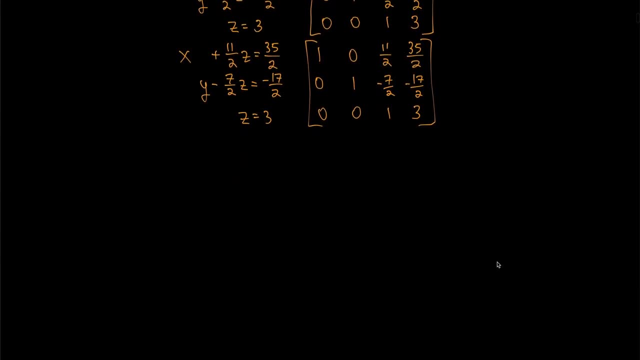 Okay, almost done. How about we now try to eliminate the rest of our z's? Because we only have one equation with x, we only have one with y, but we have three that have z in it, So I could probably do that to both of these at once. 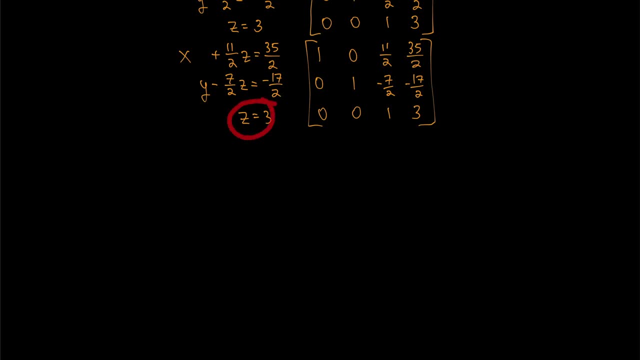 I can take this third row because it only has z in it, and I will multiply it by negative- 11 over 2, and add it to this one. That'll eliminate that z. And I'll multiply it by 7 over 2 and add it to this one to eliminate that z. 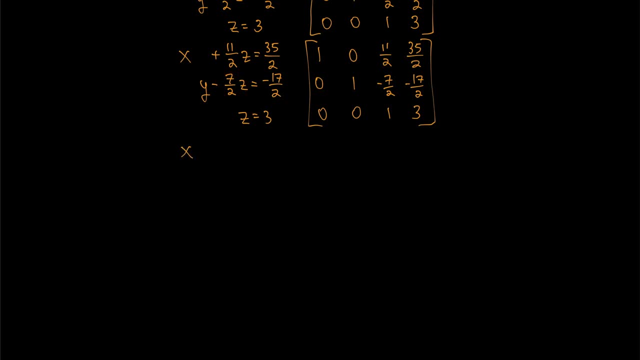 So for the top I'll just get that x plus 0 plus 0 equals 1.. And for the second equation I'll get that y equals 2 and z equals 3, which is the same as the matrix 1, 0, 0, 1.. 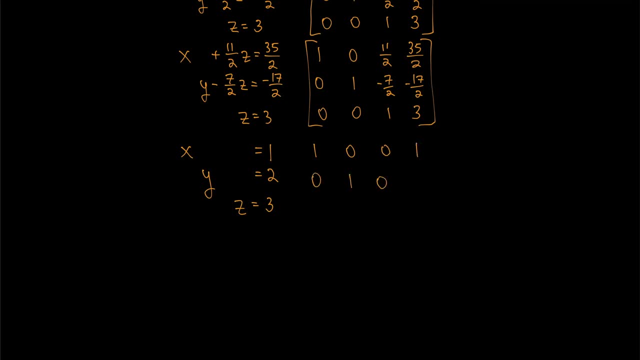 0, 1, 0, 2, 0, 0, 1, 3.. And we could also just write this using commas: x equals 1,, y equals 2, and z equals 3 as the solution. 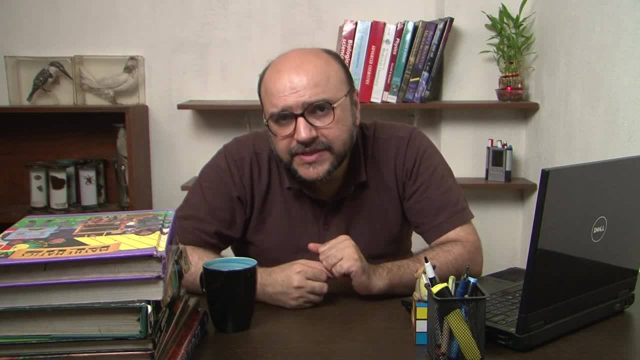 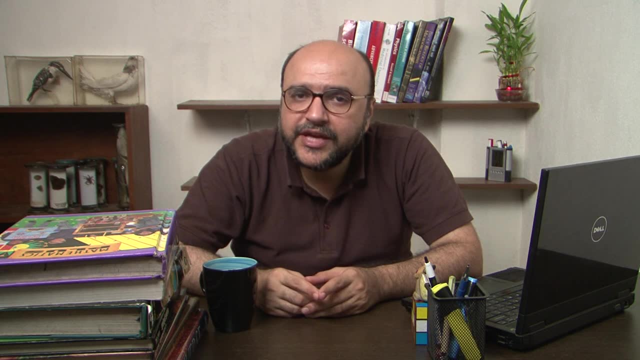 Do you know a classical piano or a harp is made of strings of the same thickness but different lengths. Frequency of a sound and pitch depends on the length of the wire being used. The more the length of the wire, the lower will be the frequency of the sound being produced, and so we get a lower. 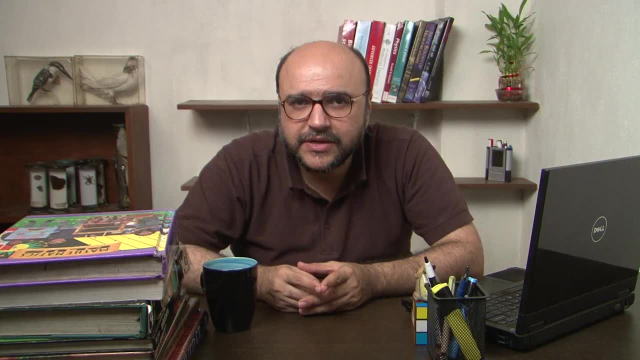 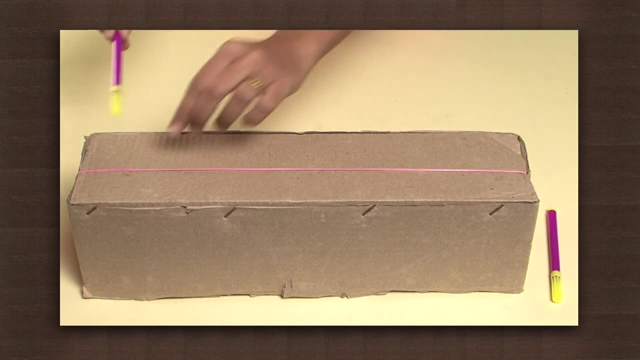 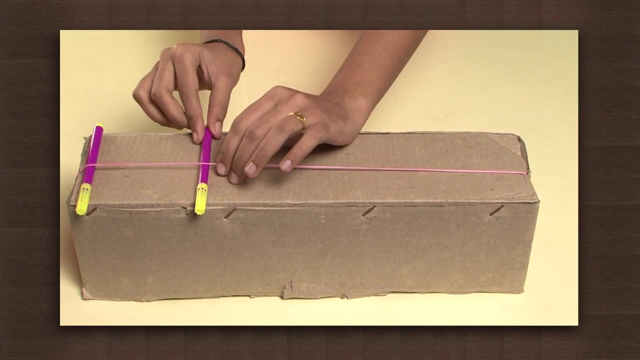 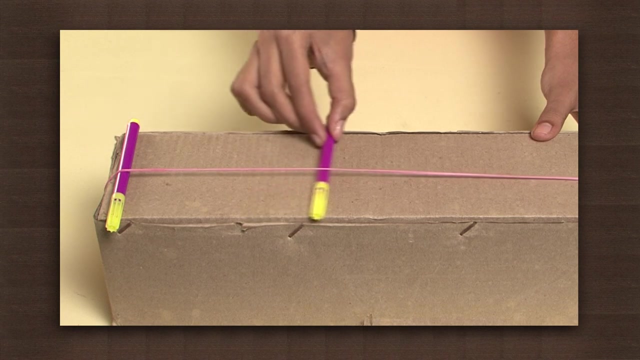 pitch. Let us try to understand the effect by a simple experiment. Here we have a box with a rubber band tied around it and two pens. Put both the pens beneath the band at a distance. Now plug the band and hear the pitch. It is sharp. Now adust the distance between the 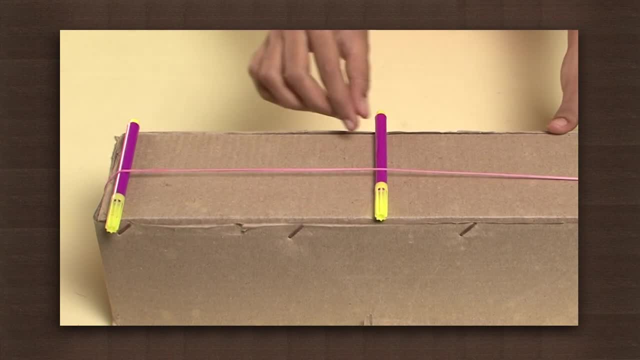 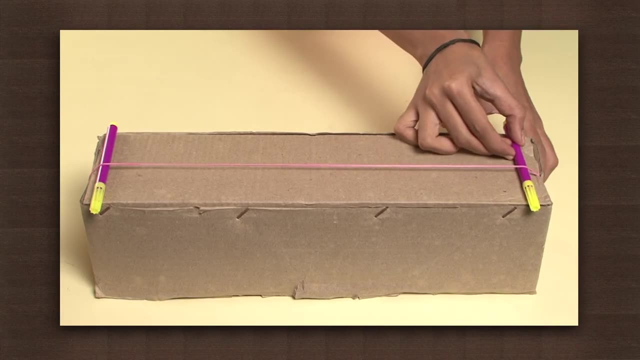 pens to increase the length of the vibrating band. Plug it and hear the pitch. You will notice a difference in the nature of the sound produced as we change the length of the string, The frequency of a sound, and here the pitch, The frequency of a sound. 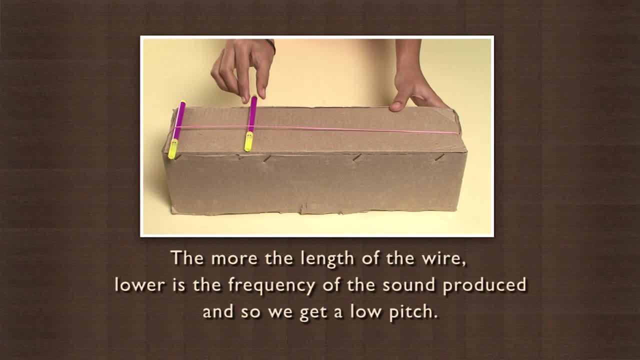 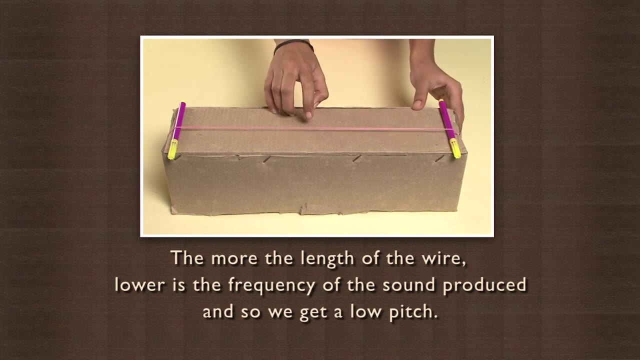 sound and pitch depends on the length of the wire used. The more the length of the wire, lower is the frequency of the sound produced, and so we get a low pitch. Wires of the same thickness but different lengths are used to make some musical instruments.